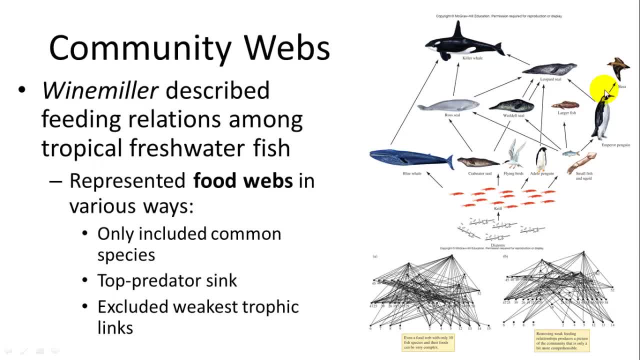 we're just going to focus on the ones that are our largest and most important and have the strongest interactions. So that's generally how you see them, But in all of them you have a sync of types. So the top predator that really, um, is very diverse in the things that it eats. 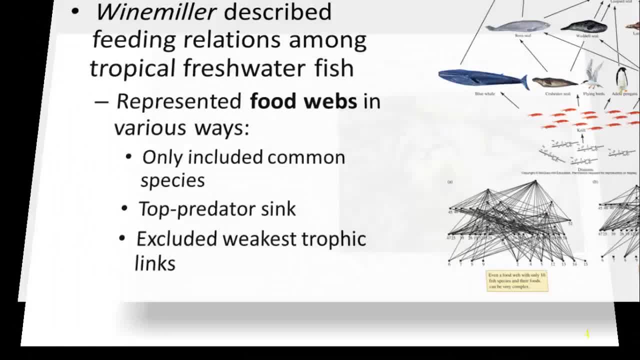 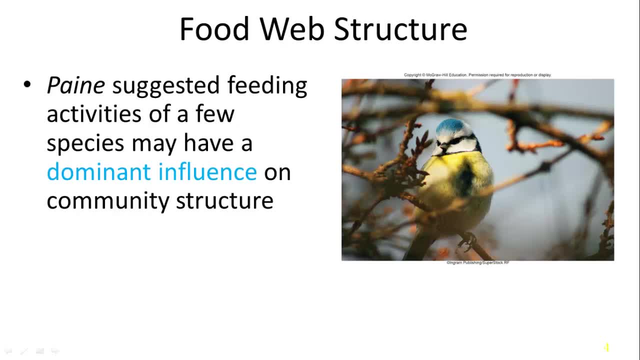 and it acts as a sync for many of the other species. So Payne then suggested that feeding activities of just a few species, those top predators, is going to have a very dominant influence. So these are dominant species in a community And the criterion for that was a strong interaction. 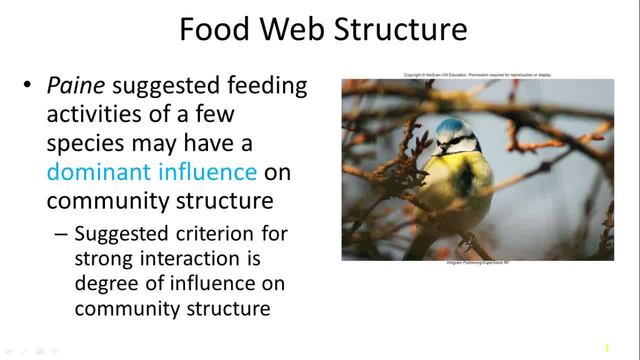 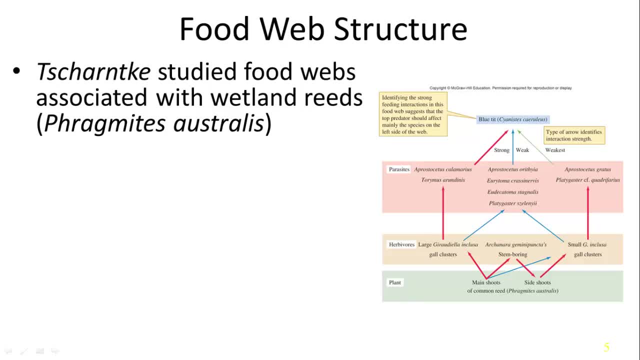 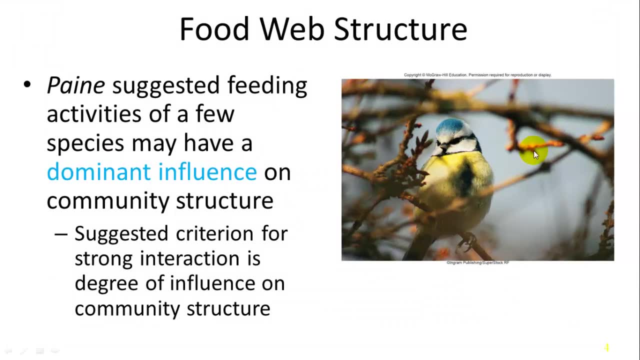 Um is the degree of influence on the community structure. okay, So Sharkey studied some food webs associated with the wetland reeds, And this isn't a wetland reed one. this is of that um buried here which is called the blue tit. 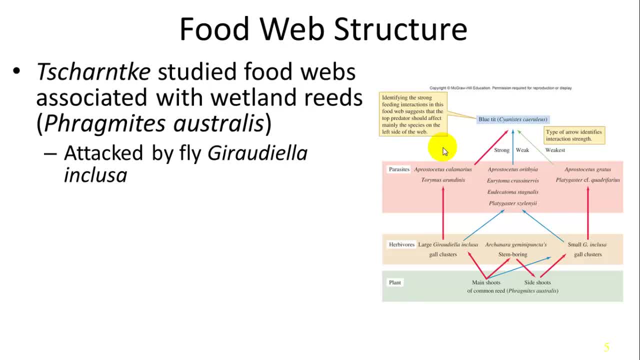 But anyway, he uh looked at this um wetland reed structure in the food web, um up and down uh, but at the base was the wetland reeds And these are attacked by a fly, which are attacked. 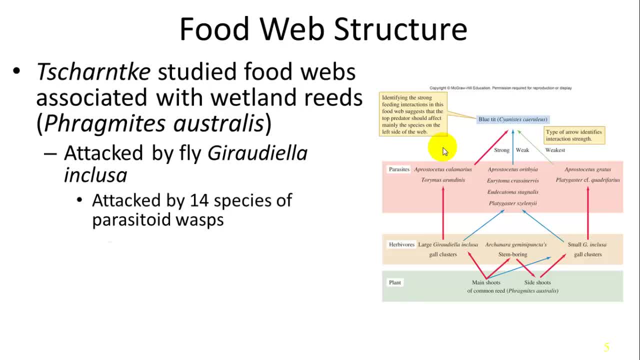 by 14 different species of parasitoid wasps. okay, And so here you have a specialization by a predator, And again he distinguished weak and strong interactions and found that some interactions were very, very strong And these could help determine what a keystone species is. 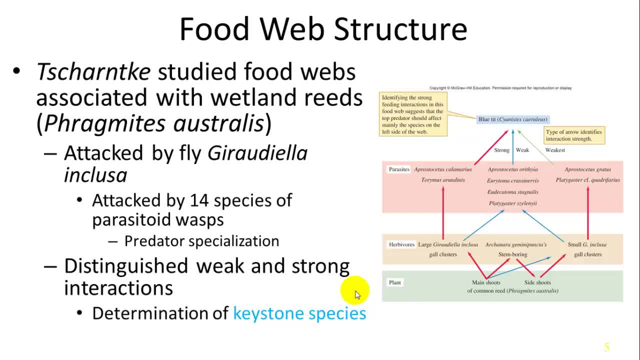 which we'll define later, But the keystone species is one that has very small biomass but has a large influence on community structure, And so what was important about the study, though, was it was able to determine strong, weak- weakest interactions and how that affected the community. 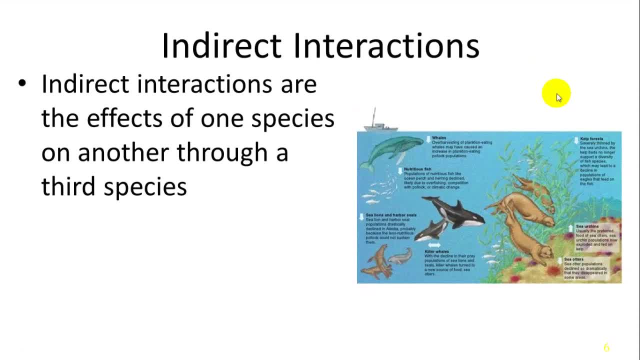 Alright. so indirect interactions are ones that usually have a third. you know you have two species that are somehow, somehow very strong connected through a third species. So an example we have are trophic cascades, indirect commensalism and apparent competition. So we'll talk about just. 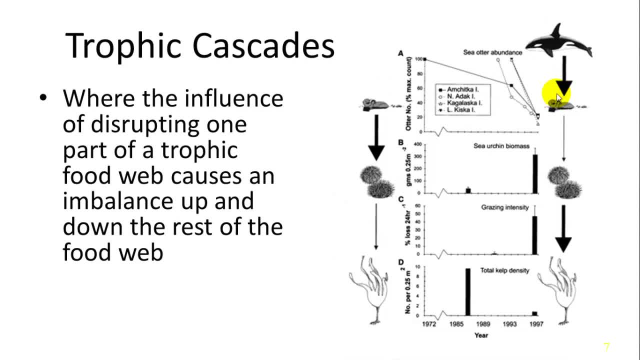 briefly about trophic cascades, which is basically where the influence of disrupting one part of a trophic cascade or trophic food web can have effects up and down the rest of the food web. An example of this is killer whales- Killer. 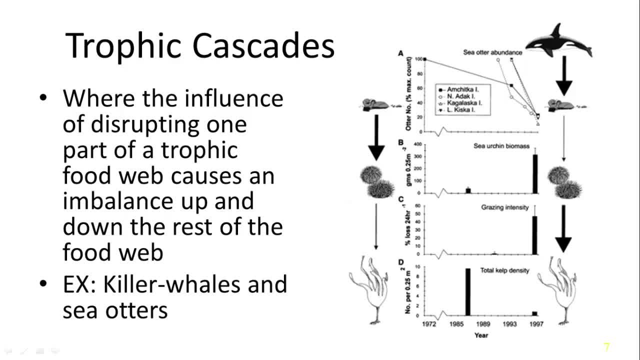 whales don't normally feed on otters. They normally eat seals and sea lions and stuff, But recently they've started to eat more of these sea otters. It's part of made a more significant part of their diet. The problem with that is that 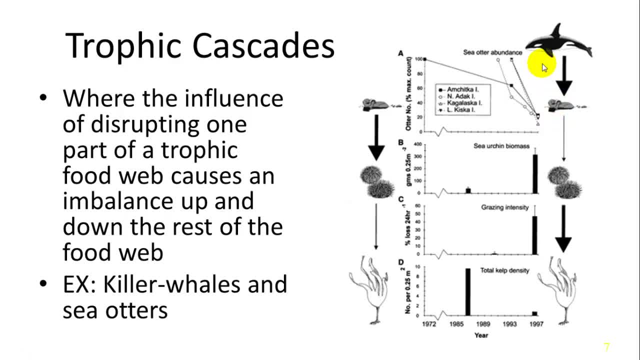 well, the reason why that is maybe a couple different reasons, but seals and sea lions are reducing in number, partly because of, perhaps, overfishing by humans, And so they aren't as abundant, And so the killer whales have to find another food source, And so they start eating these sea otters. Well, the 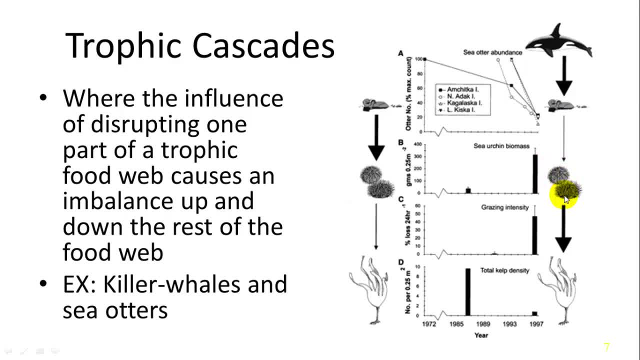 sea otters eat a lot of echinoderms, such as, you know, sea stars and these, the other echinoderms- I cannot think of the name right now, But anyway, these sea urchins are there. Yeah, sea urchins. 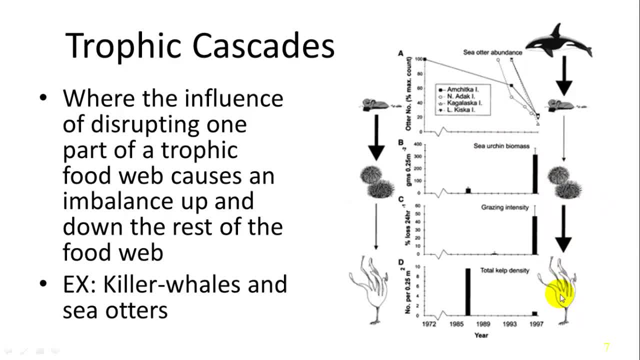 And sea urchins are grazers, They eat kelp. So if you eat too many of the sea otters, the killer whales, it will cause an increase in the biomass and production of urchins, And that will then increase the amount of kelp predation. or 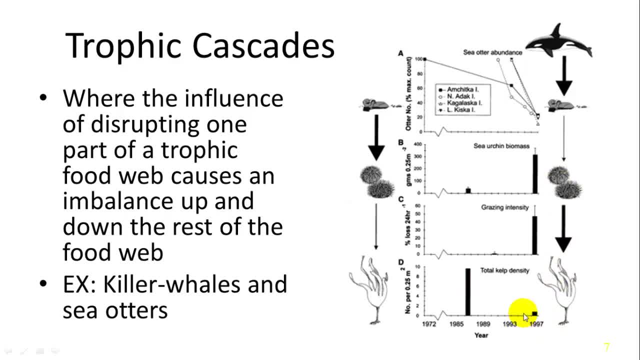 herbivory by the sea urchins, And so kelp will be significantly reduced And that's going to significantly reduce the amount of kelp And that's going to significantly reduce many other species that use the kelp for food and for shelter and such. So just 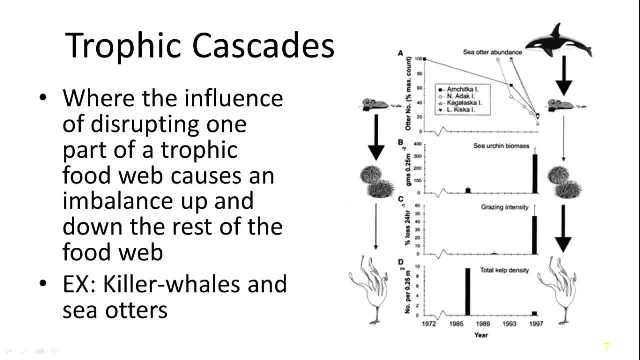 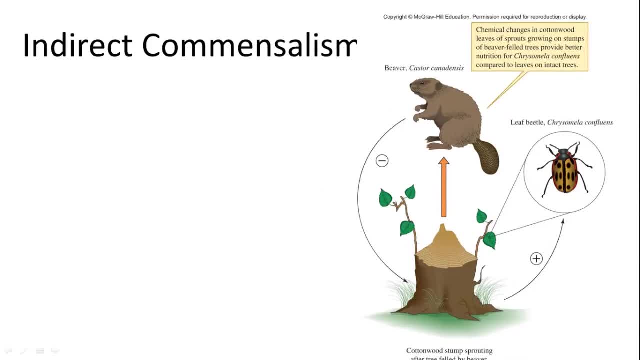 by affecting one part and you have a trophic switch. you can have a cascade of effects, All right. Indirect commensalism is where one species indirectly benefits another, while through a third species, while the other one is neither help nor harm, So it has a neutral. 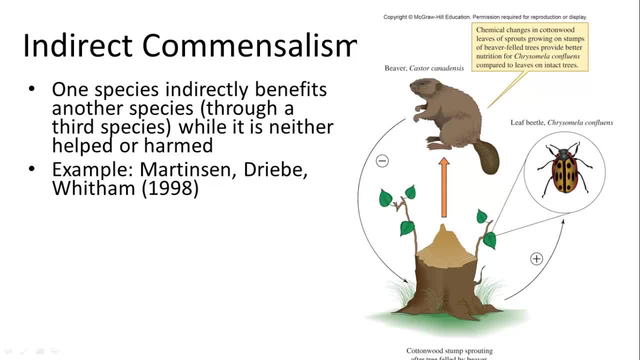 relationship. So the example was discovered by Martinson, Dreeb and Whittem. Beavers will cut down cottonwood trees, you know. chew them down And in place of their trunks you will get seedlings to pop up. Beetles like these seedlings because they're high in nutrients and easier. 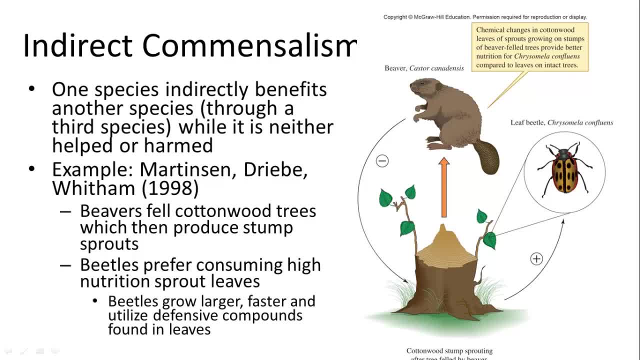 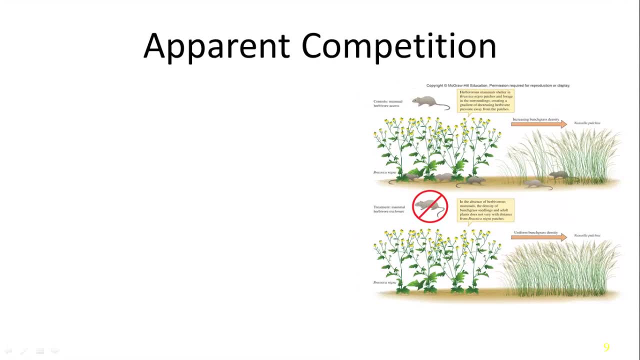 to eat, And they grow larger and faster and just reproduce better. So a beaver, then, positively benefits this beetle through a third species, the cottonwood species, while not negatively affecting itself. All right, Our parent competition is the third one. This is where negative effects between. 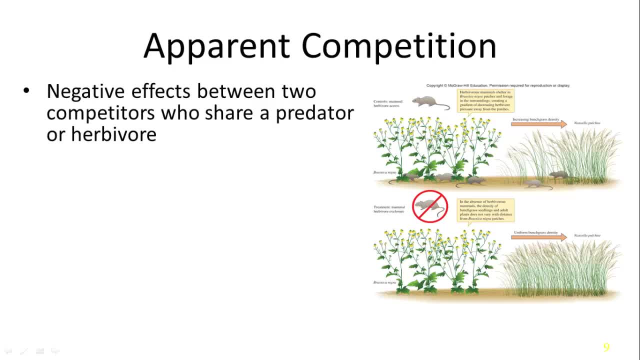 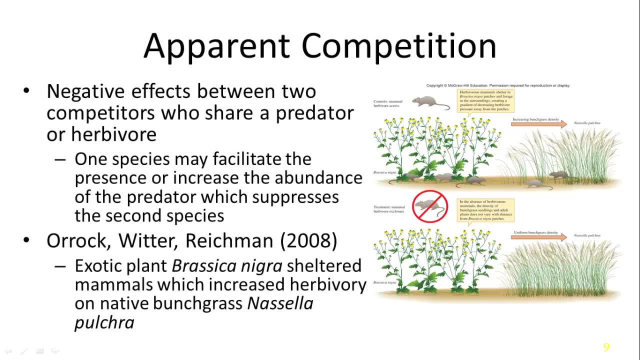 two competitors who share a predator or herbivore. So one species may facilitate presence or increase the abundance of the predator, which suppresses the second species. Orock, Whittier and Reichman in 2008, they looked at this exotic plant, Brassica nigra. 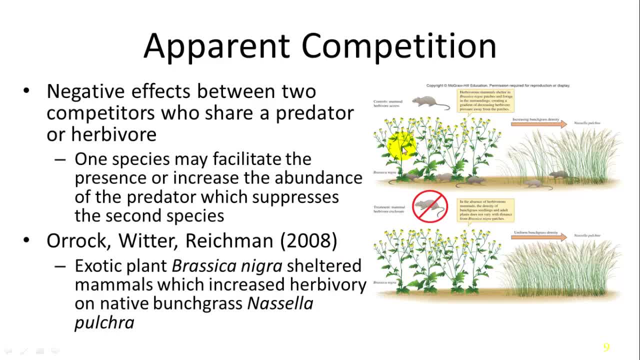 And they found that it was not native to them. So it isn't originally there And it shelters small mammals And then, by sheltering these small mammals, they will spend more time there And so these bunch grasses which are native to them, they found that they will increase. 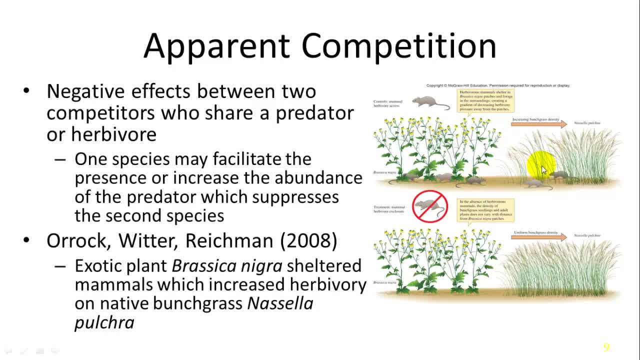 in density as they get further and further away from these sheltering plants, Whereas if you don't have the mammalian species, the bunch grass species will have uniform density. Okay, So this apparent competition, it's not actual competition between these two plants. 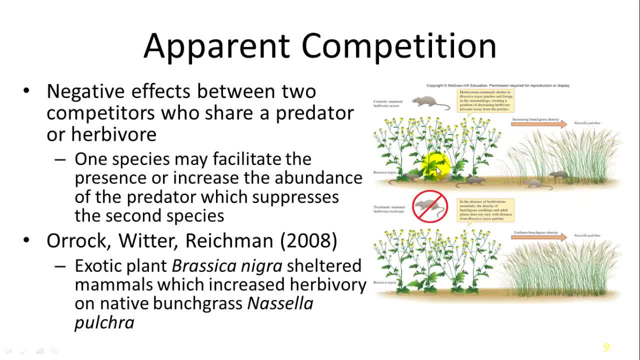 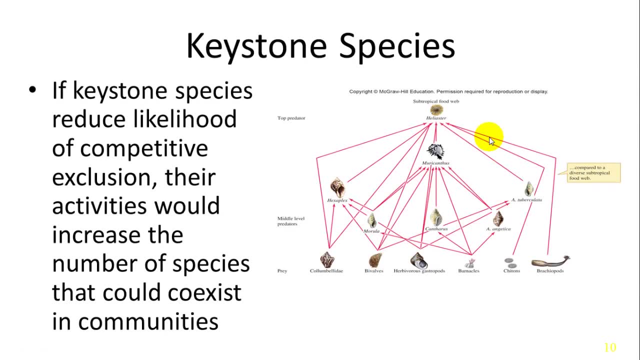 But because this one plant is housing the mammals, that mammal's mammal then decreases the abundance of the other one, So it's not directly competing. They're apparently competing, All right. The keystone species again is one that has less biomass and great influence. 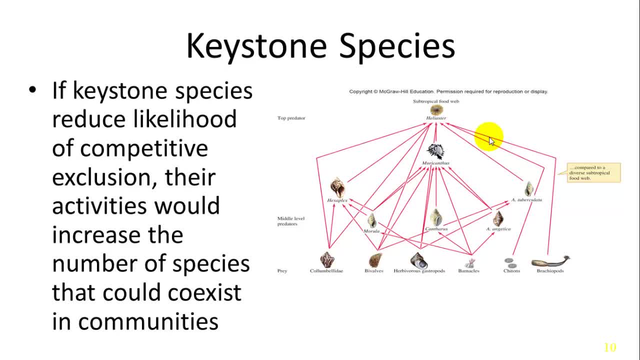 If keystone species reduce likelihood of competition or competitive exclusion, their activities would increase the number of species that could coexist in communities. Okay, So if it's a predator, this keystone species is a predator. it might keep other populations in check so that competition doesn't over-exclude other species. All right, So looking at food, 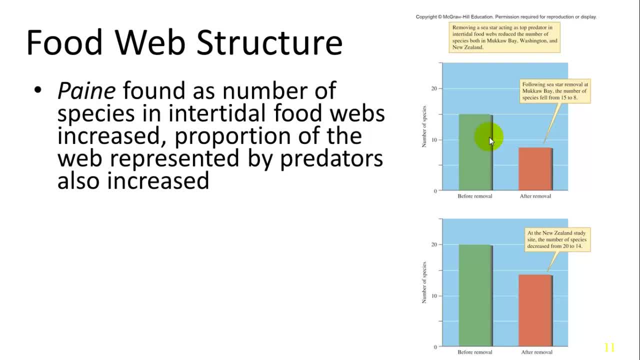 web structure. Payne found that as the number of species of intertidal food webs increased, that more of the species were represented by predators. So a higher proportion of predators produces a higher predation pressure on prey populations, in turn promoting higher diversity by removing those that would normally exclude others by competition, And he found this with 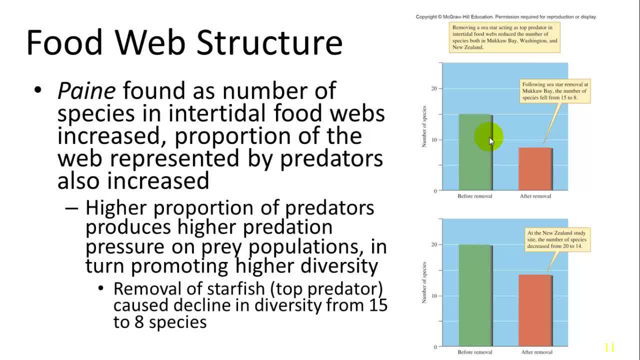 the removal of species Starfish. Starfish are a top predator. They eat out lots of mussels And they keep then populations in check from competing each other. So when you remove these species you have a significant reduction in species. So this is a keystone species. 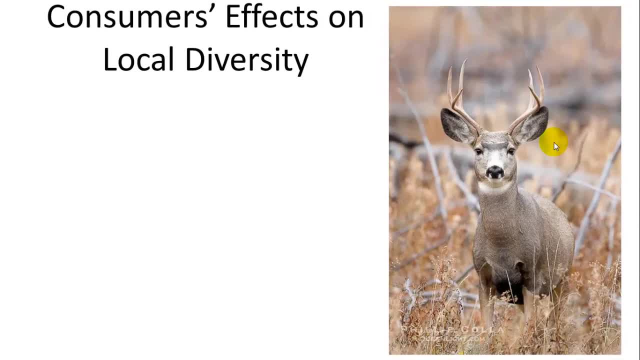 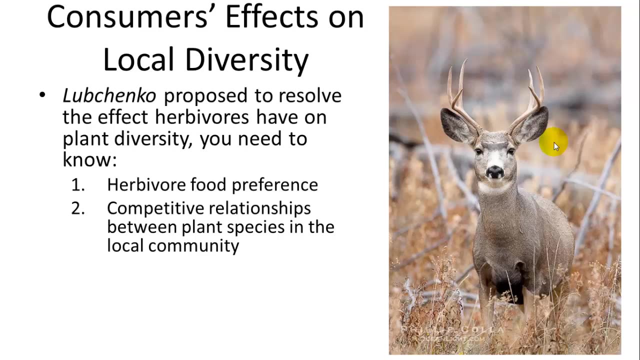 All right. So some consumer effects on local diversity. Well, Lubchenco proposed to resolve the issue of herbivores on plant diversity. You have to know three things. One, what's the food presence of the herbivore? Second, what's the competitive relationship between? 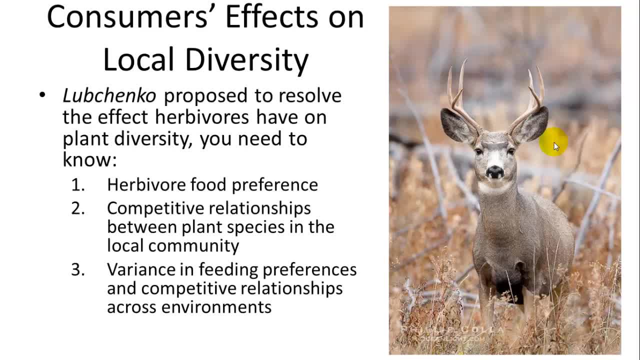 plant species. And third, what's the variance in feeding preferences and competitive relationships across environments? So kind of both. So, really, if this deer prefers one grass species over another and that grass species is out-competing other grass species, so you know the food preference. 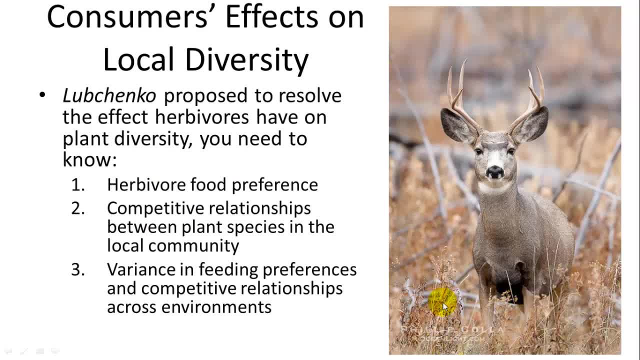 of the deer. you know the competitive abilities of this species relative to other species, then if this deer is eating this species, maybe it's keeping allowing the diversity of other, less competitive species, And you may then look among different environments to see if that same relationship exists. 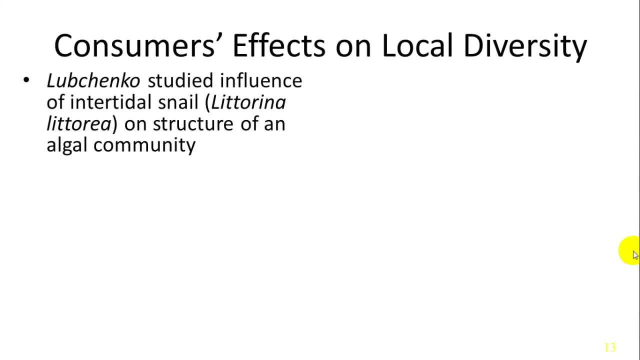 All right. So Lubchenco studied influential intertidal snails. So another intertidal study. He looked at this snail on the structure of an algae community. Snails are grazers on algaes. So we have two species of algae: red and green algae. 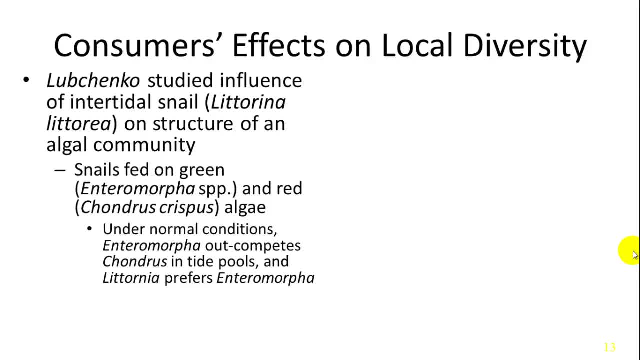 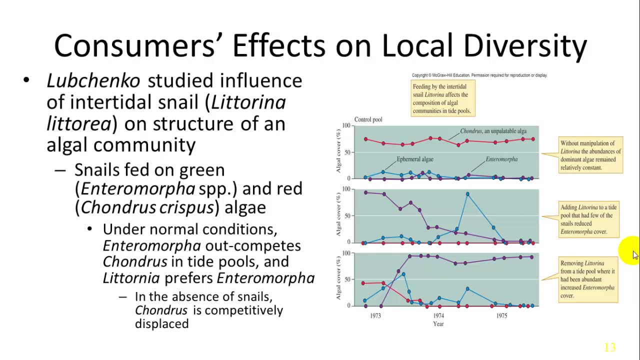 And under normal conditions, Enteromorpha, which is the green algae, out-competes the red algae And the snail prefers Enteromorpha. Okay, So in the absence of snails, the red algae is not around. It's competitively excluded. 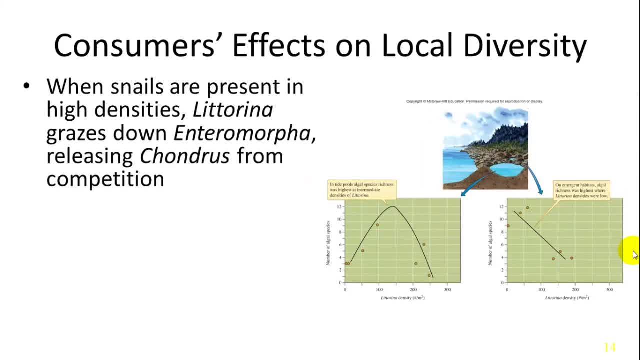 by the green algae, But when snails are present in high densities, okay, a Litterina grazes, it prefers the green algae and then releases Connors from competition, So then it can also colonize those areas. Green crabs are a mechanism for reducing the snails, So they will prey on young snails. 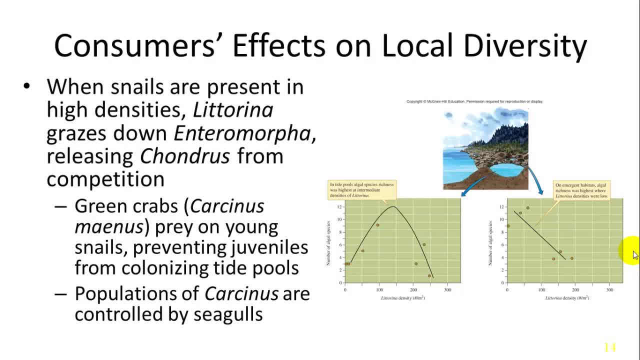 and prevent juveniles from colonizing the tide pools, and populations of carcinous are controlled by seagulls. So here we have trophic effects. here. If you have crabs and seagulls, Okay, Okay, Okay, Okay, Okay. 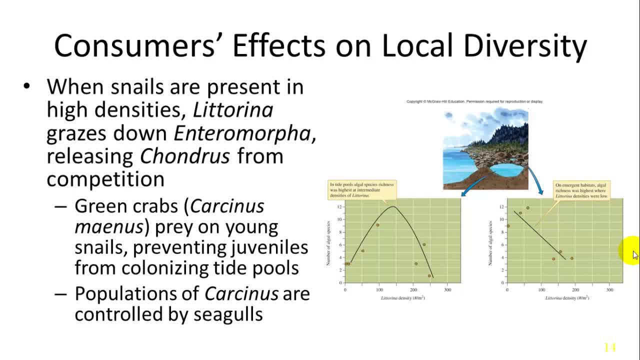 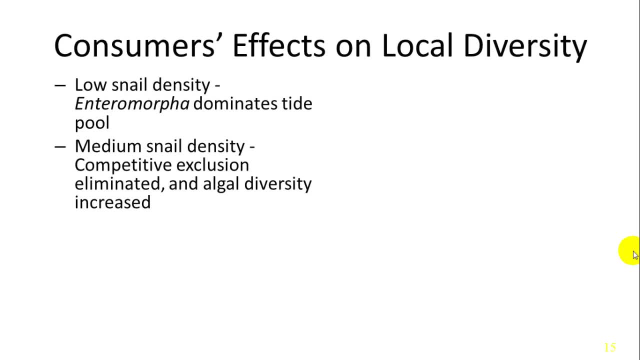 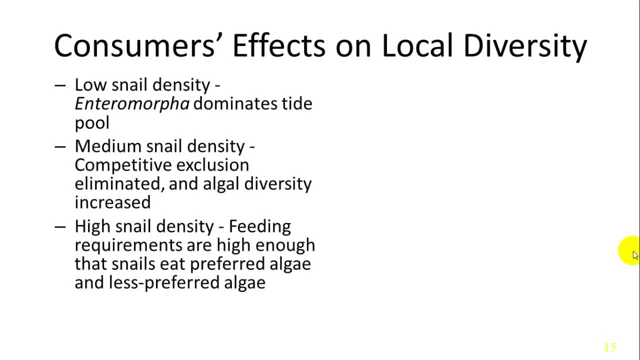 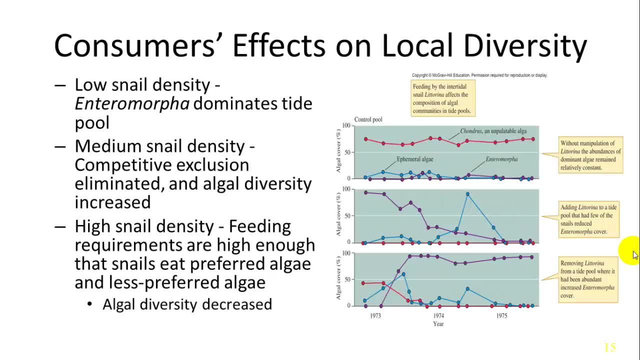 In high snail density, the feeding requirements are high enough that the snails will eat well both of them, and so they will both be reduced significantly. okay, and these are the graphs showing that. so here's your two algae species and this other algae which isn't eaten at all. 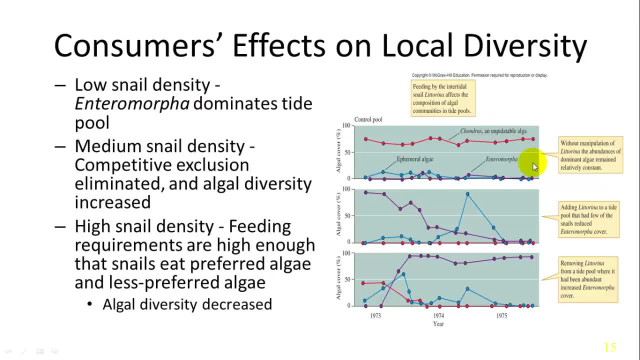 okay, and if you have a snail in there, it's gonna eat these algae and that one's gonna be just fine. okay, the unpalatable one will increase. but if you decrease the, if you increase the amount of snails, this unpalatable algae will be decreased significantly. 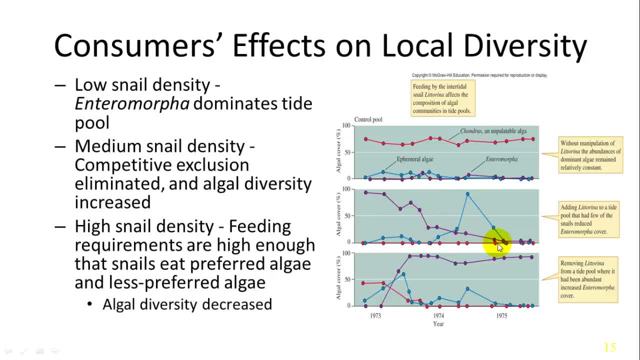 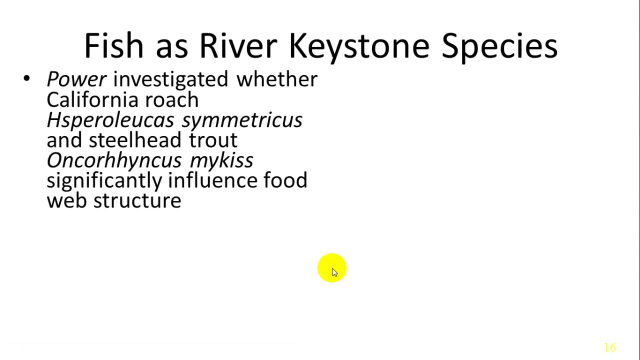 because these two species can out-compete it. and then again same thing. and when you remove these snails completely, again that red algae will decrease significantly and one of them will out-compete the other two. so competitive exclusion. alright Power also looked at whether this a couple different species of fish. 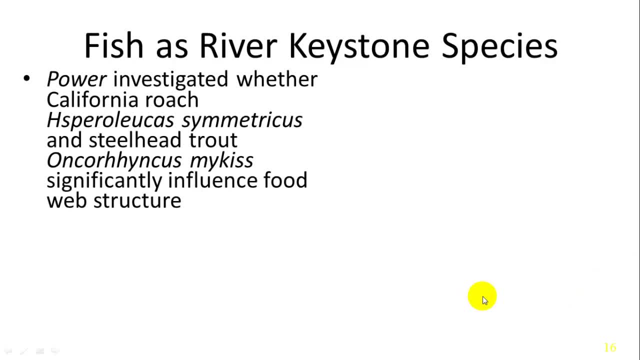 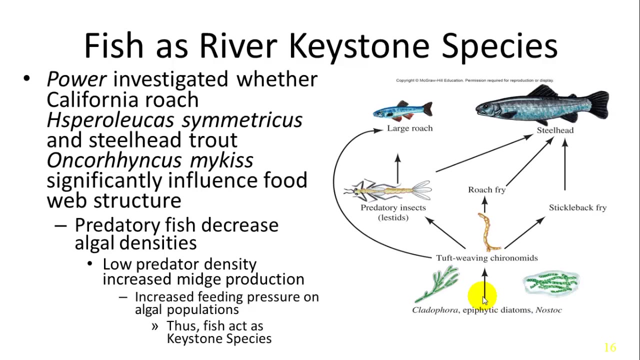 significantly influence food web structure and predatory fish decrease algae densities. a low predator density increased midge production and that increased feeding pressure on algae populations. so this fish acts as a keystone species. so again, if you have predatory fish, they decrease algal densities by low predator density. 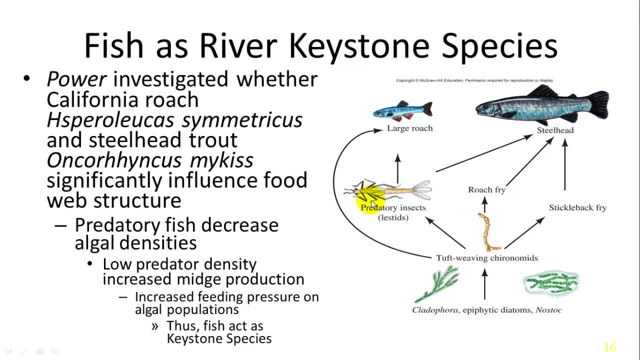 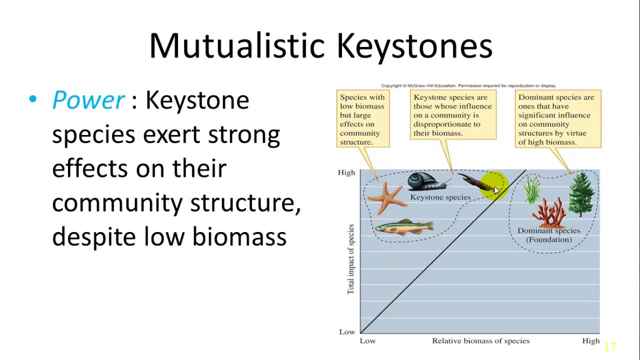 increasing these midge productions. okay, so they're eating these midges and these midges eat the algae. so even though they're only eating one part of the food chain, they're going to increase. they have an overall effect which is higher. so again, Power. the keystone definition is 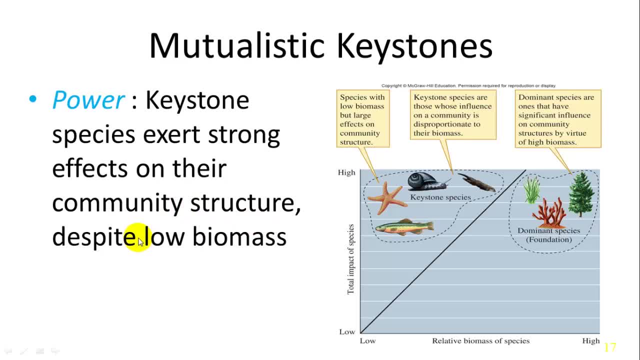 species that exert strong effects on the community structure despite low biomass. when you look at it graphically, you have these keystone pieces who have biomass, which is low, but their impact on the community structure is low and the environment is very high. dominant species, on the other hand, 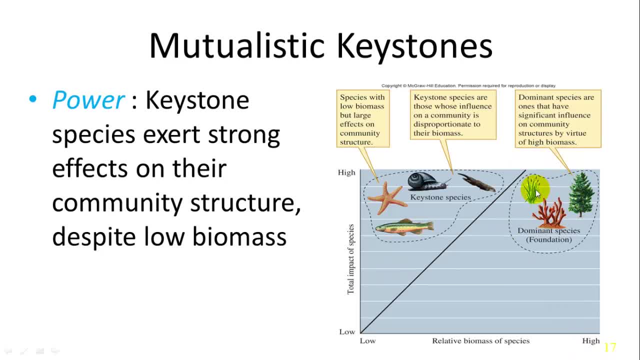 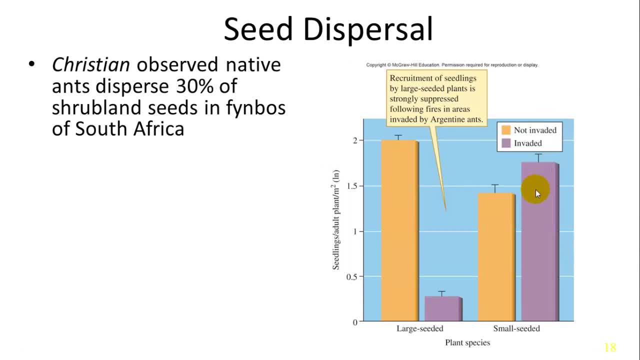 have both high biomass and high impact. okay so in seed dispersal, Christian observed native ants disperse 30% of shrubland seeds in the fin boats of South Africa, so they're very important for dispersal. there's mutualistic association there. they get food.